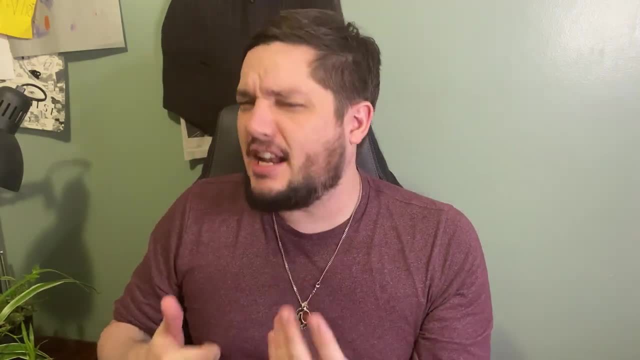 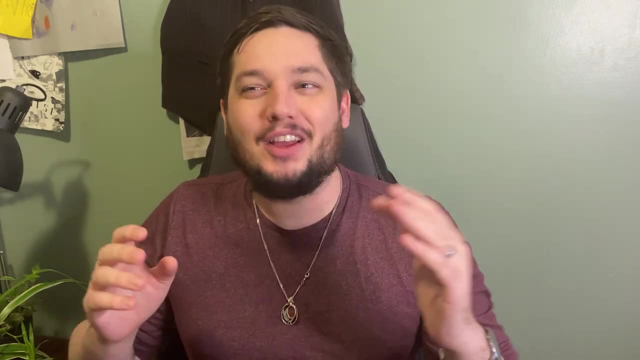 Seriochemistry is one of those topics with inorganic chemistry. that, I think, is part of the reason that the topic gets such a bad reputation. People find it really hard, I think, to visualize these structures in their brain and be able to tell whether it's an R or an S, or appreciate. 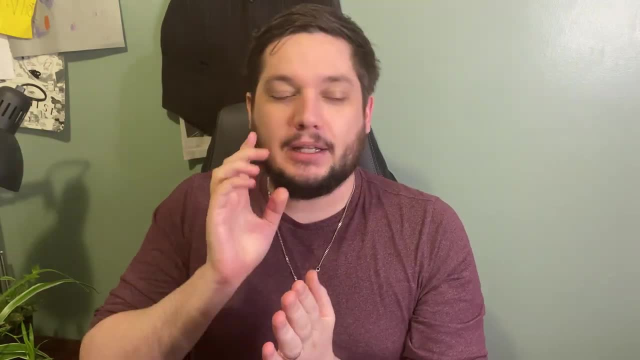 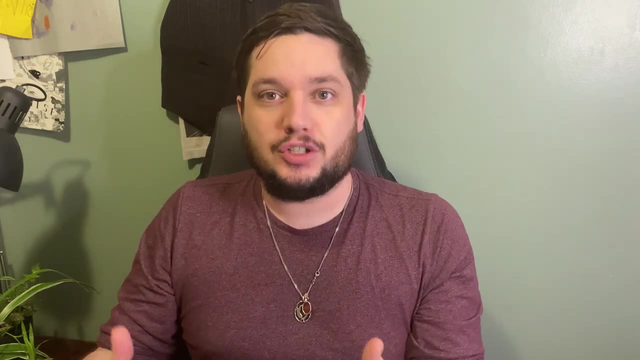 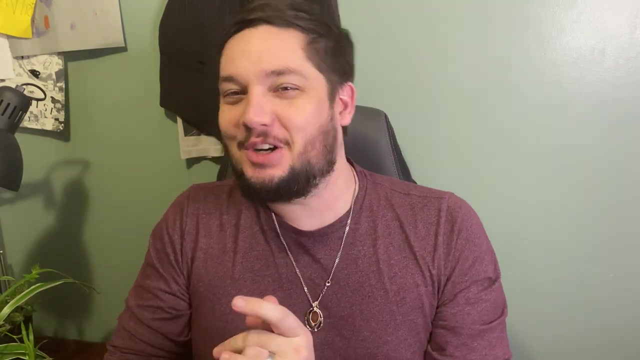 the difference. It can be really hard to keep things straight, But luckily ChemSketch has some tools in it that is really helpful and to enhance your studies and be able to visualize things much more effectively. Hi, I'm Jesse. I'm a marketing communication specialist here at ACD. 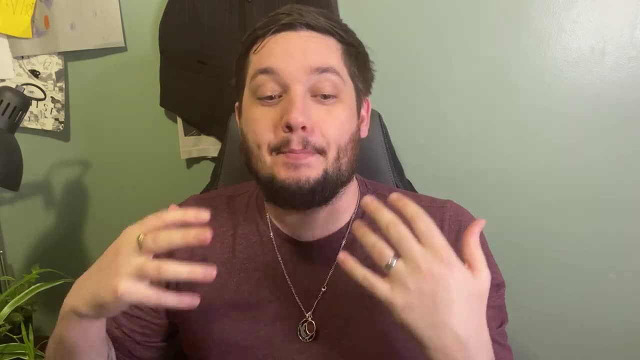 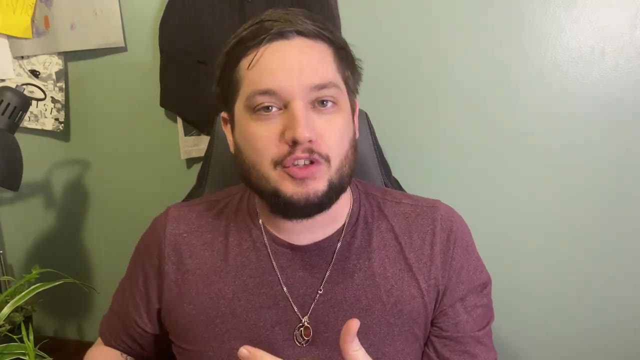 Labs And I want to talk to you today about seriochemical tools in ChemSketch. There's a lot of options in there. It's really helpful, particularly if you're somebody who's struggling with this and some of your organic chemistry homework, And I think that these tools can make 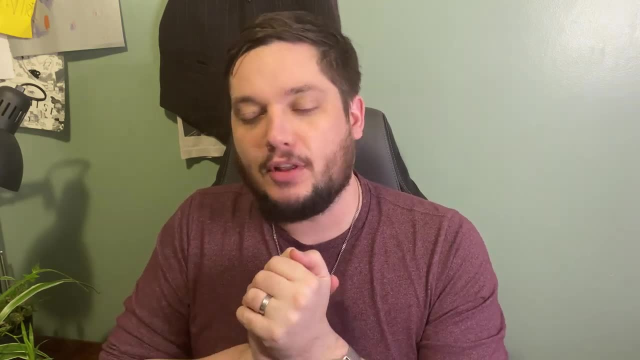 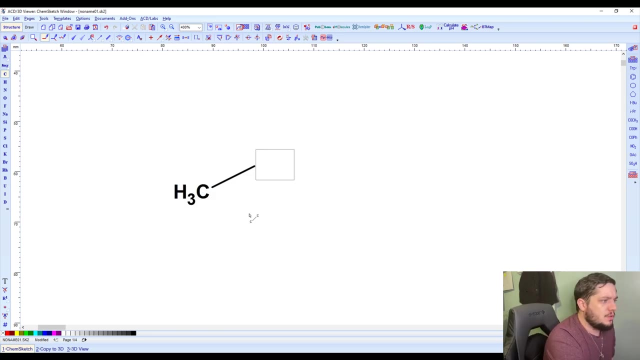 these things much more Understandable, much more approachable. So let's get right into things. Okay, so let's go through some of the most basic tools to begin with. So first we're just going to do a simple carbon carbon bond with some hydrogens here, And there is of course, no chirality here, But we have the 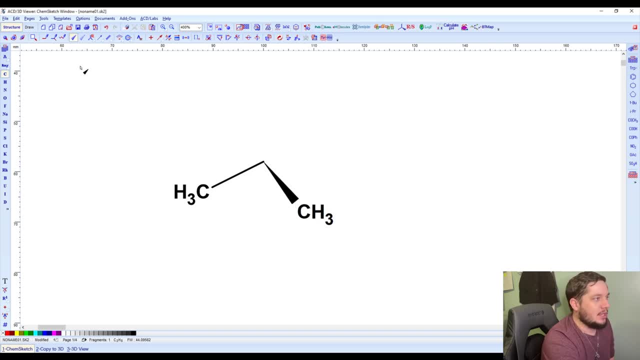 up stereo bond tool that it can be accessed through this part of the panel. By the way, this area right here is where we're going to do most of our work today. This is where most of the stereochemistry related tools can be found. Then we have the down. stereochemistry, And then we have the up stereochemistry, And then we have the down stereochemistry, And then we have the down stereochemistry, And then we have the up stereochemistry, And then we have the up stereochemistry, And then we have the. 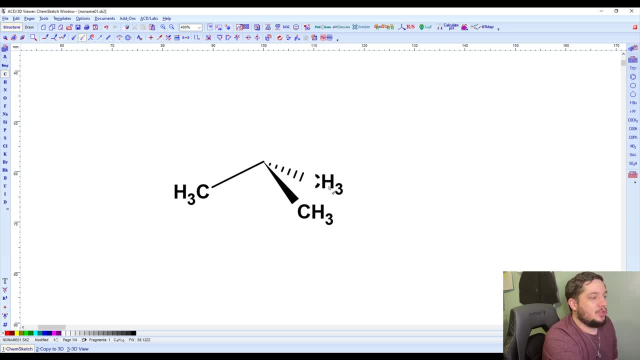 bond tool right here that shows the hashed bonds. This is the bold one, This is the hashed one, And then we can go back to our normal bond right here. So this is our little 3D configuration. Obviously, this is in chiral at this point because they're all the same atoms in every. 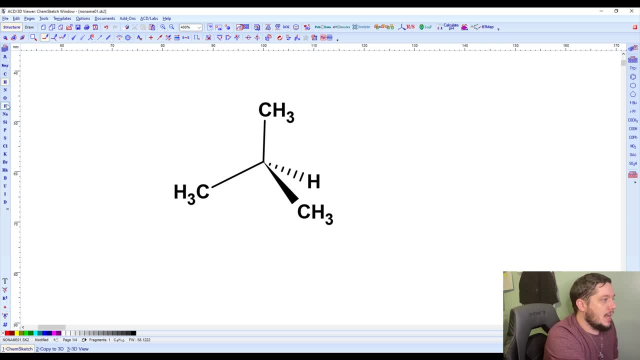 direction. So let's add in a hydrogen here, an oxygen here and a fluorine here, And then we- And this is, of course, the most obvious and most simple way that you can create a chiral molecule, And this is probably what most people will be doing most of the time. 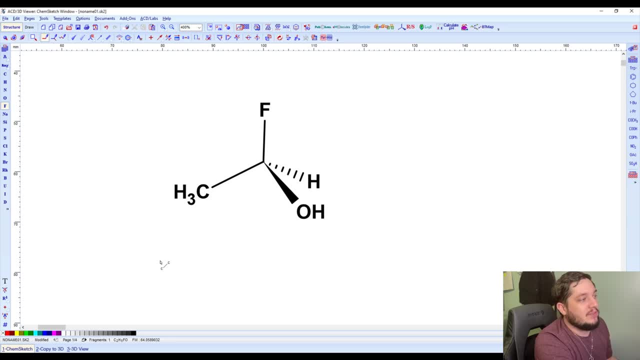 But this is, of course, ChemSketch, and we really believe in giving you a lot more tools than what you need for those simple applications, but go into the more advanced ones in addition. So one of the ones that we have here, for example, is the undefined stereobond. 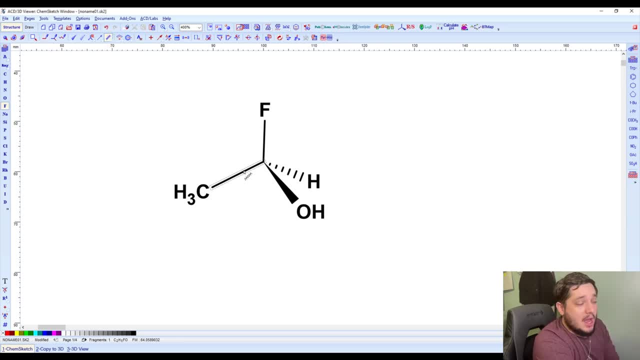 And here that if you're, for instance, working on some sort of like natural products project, this is something that you can use to show that there is some stereochemistry in a given location, but you don't exactly know what it is, For example, not used all the time, but something you have access to. 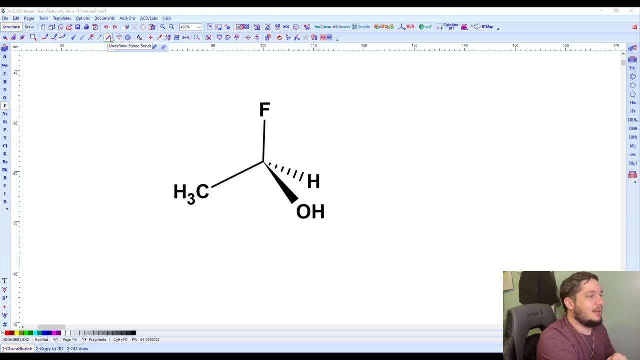 There's a few other more exotic bombs that are being hidden in here too, that if you want to use those. One that is really useful, though, for I think a lot of people, is the set2r and set2s configurations. 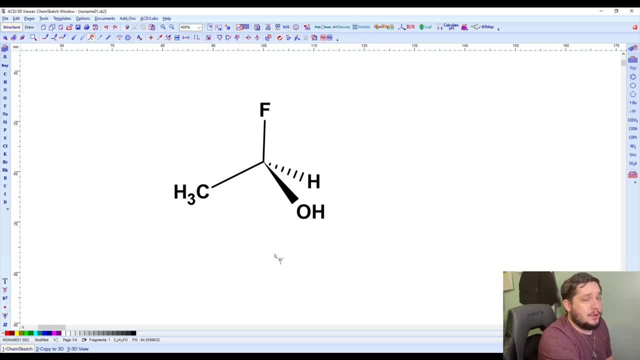 Maybe you know, Know that you want to have an R molecule, but you don't know whether this is R or S off the top of your head. You go to the set2r and you can click right here and it will set that as the R configuration and that you can see that you know they're in the way that this is laid out. 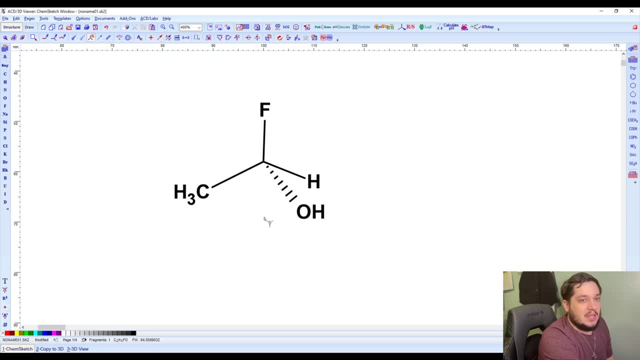 You can have set2s as well. So that also is giving you the correct configuration. here The OH is going into the page and then that's how this would be laid out here. So that is something that you know. And then Also you can use this button to generate the stereo descriptors. 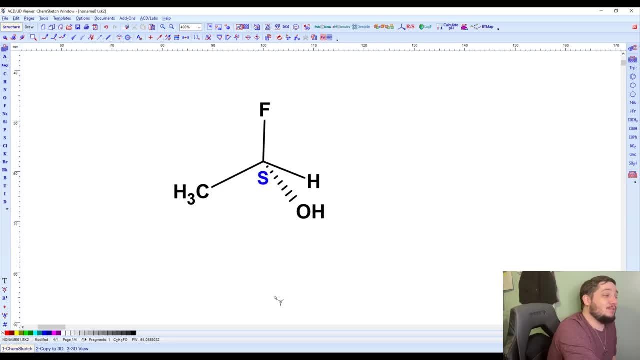 So you press that and it tells you that it's an S configuration as of right now. So that's really easy that you can, you know, do. that is, if you have a particular structure that you need to fight the route, whether it's R or S, you just draw it in here, click that button and you have that little blue S that pops out and will tell you what is going on. 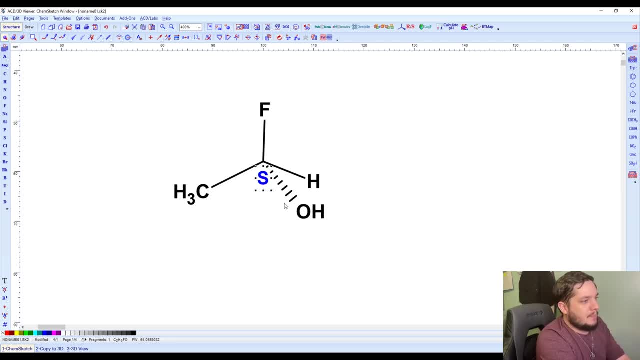 Something to note, though, that The I often use The clean structure button to clean the layout of a molecules that I create in ChemSketch. One thing to note, though, is that it doesn't really work that well for 3D structures or stuff that has a stereo chemistry that's associated with it. 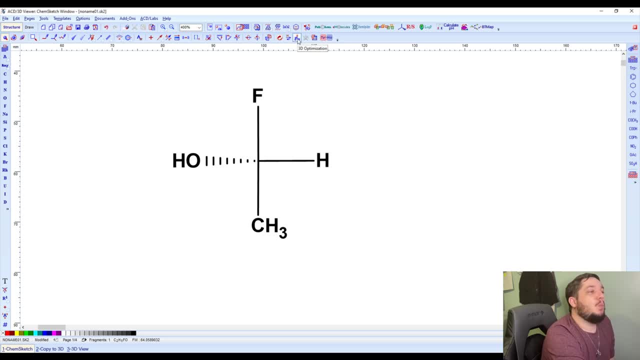 It often kind of looks a little bit wonky like this, But one thing that you can do is use 3D optimization with room. Yeah, this comes up to worry about it here. So, yeah, you get a couple of warnings That that pop up. this doesn't look as nice in two dimensions, but when you start moving it around in using the 3D dimension mover, you can see things a little bit more clearly and you can eventually maybe try and get into a configuration that kind of shows: uh, you know what you want. 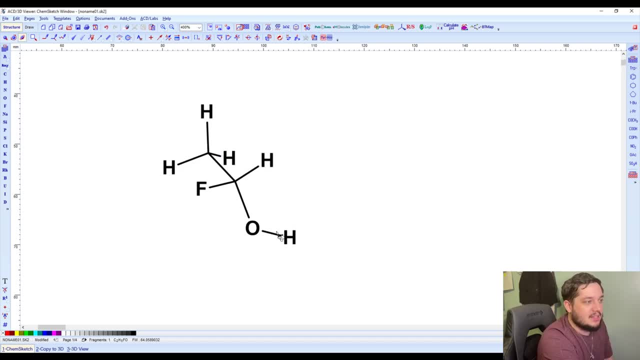 Um, that's actually not a bad one. right there You can kind of get a bit of a sense of the 3D feeling for it, but I I find that the, the actual sort of moving around itself, is the easiest way to visualize it. 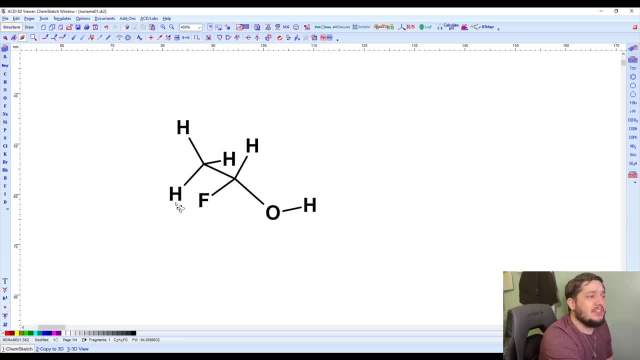 We're going to see a more Advanced version of that in a little while, But this is a really useful way in kind of like everyday use, and that you can turn around um fairly large molecules in this and get a view of how things are laid out. 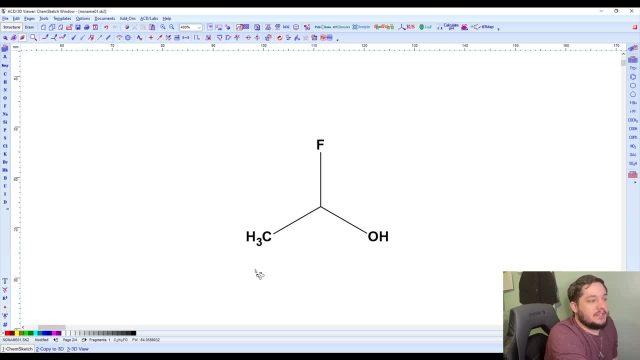 Um. now, beyond this, we have some other uh options in terms of laying out different molecules. Um, we can, for example, this layout as of right now: um, everything looks flat. Um, but we can actually use this too. 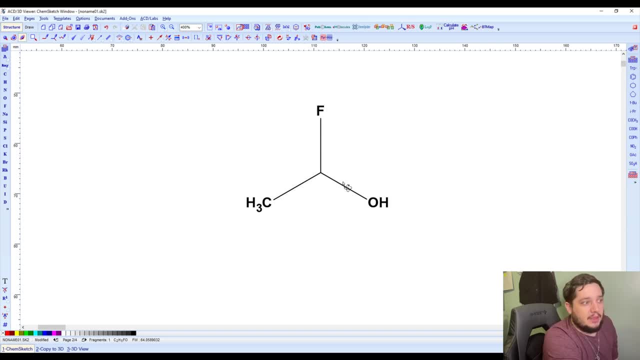 Um, you know, see the uh, you know names of the molecules as well and and determine the uh stereo chemistry that way. So we can click here, generate name from structure. Um, this one, of course, is not, you know, chiral at the moment. 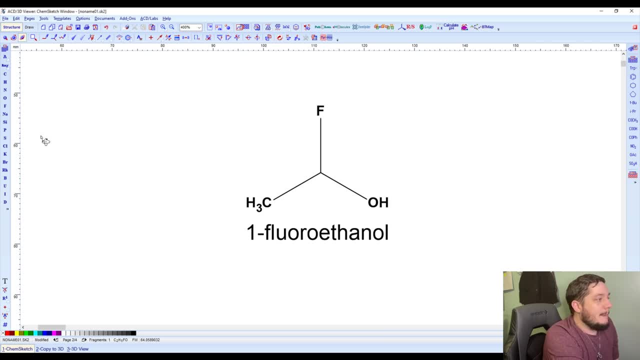 Um, it's not seeing any chirality here, so that's why we don't get anything there. But if we go back, we can pull out the down stereo chemistry there. Uh, let's change that to a hydrogen so that it's actually chiral here. 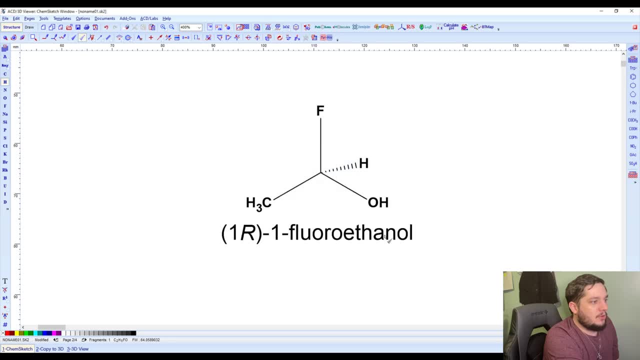 And we can then generate name from structure and we have that R that's given to us here. so that that is, you know, we know that now this is an R configuration of the molecule. We can change the, the structure, uh, and have things. um, actually, let's do it with um, this one here. 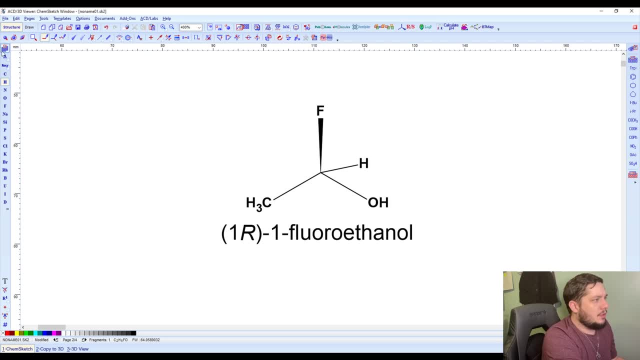 Maybe we show that one is flat, Um, something along those lines. I don't know if that'll flip things, but let's generate a name based on that. That's R once again, Um, but let's actually, let's actually try and, uh, flip it around. 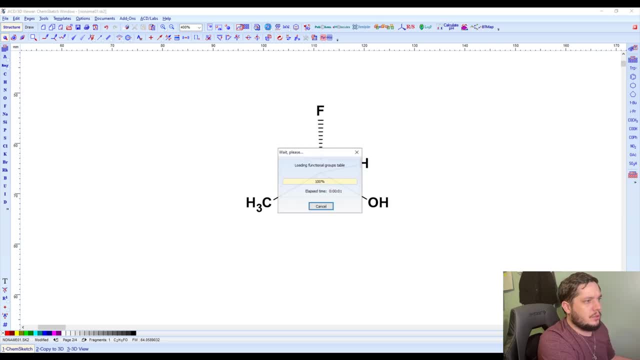 So, yeah, so it'll update when you, when you change it. Um, now, if you are just changing the structure of the name won't update automatically, uh, as as you're changing it, but you can always regenerate the name and get one over top of it. 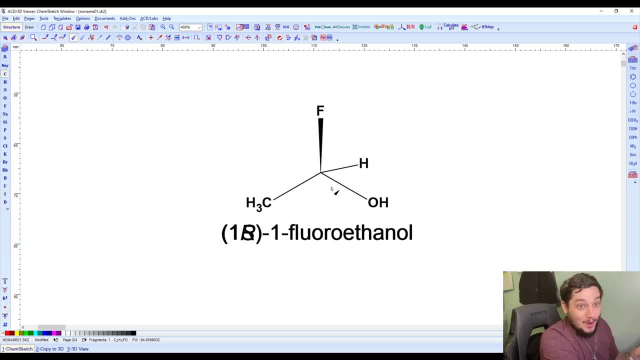 Um, but so, yeah, you just create them again and again. So that's just something that you should be aware of as you're, as you're doing that, And it's not going to be fixed, you know, Over over time. 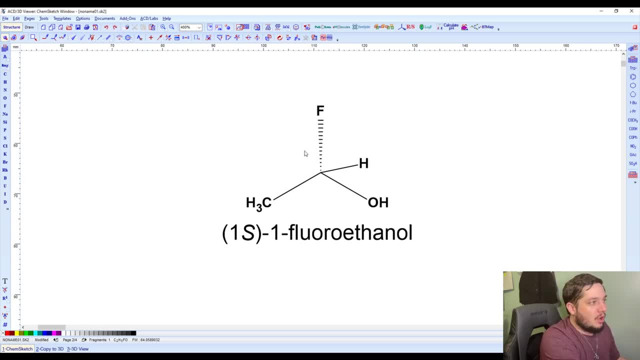 Anyway, that's something to be aware of. Now, there are ways in which you could display things and it'll sort of confuse it, Um. so, for example, let's do a little mistake, Uh, let's do this one right here and create a name for this, and yeah, so, incorrect configuration definition. 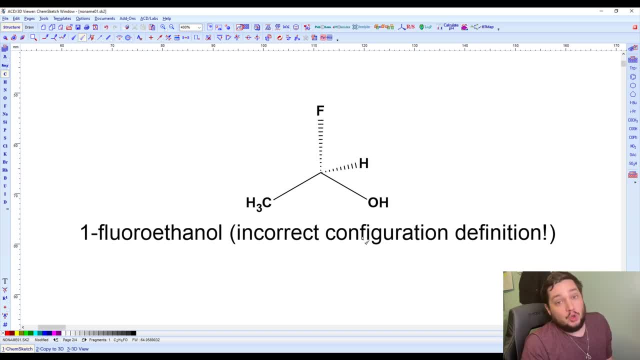 So basically, what this is telling us right here is: it doesn't know what stereochemistry we're looking for in this Cause. this is obviously like we have two of them that are going into Yeah The page, So it's a little bit unclear. 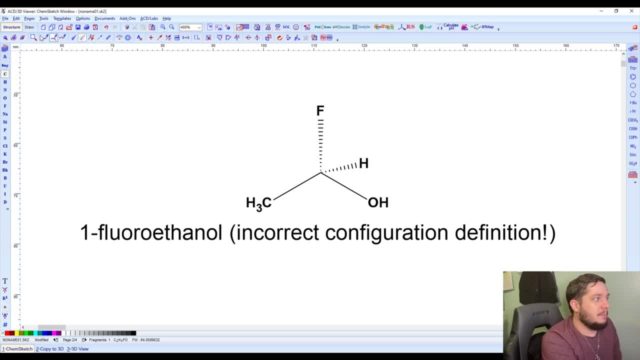 Um, but this is something that you, if you're getting this um configuration, if you're getting this, this warning, maybe try a different configuration, sort of move things around, uh, and you might be able to get um a better answer. 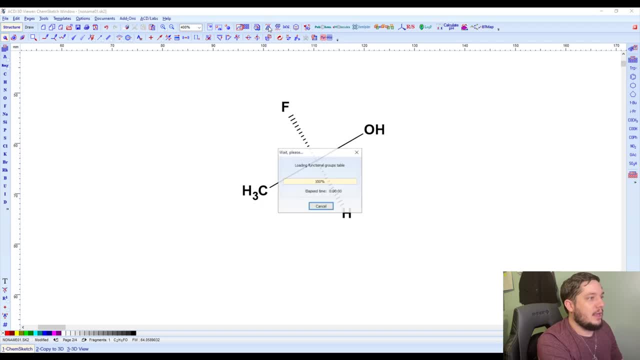 So let's go here, Let's do that, Uh, and then let's generate a name right now. Okay, Now it's figured something out for it. So there's the. it'll be able to tell a lot of it. It'll try its best. 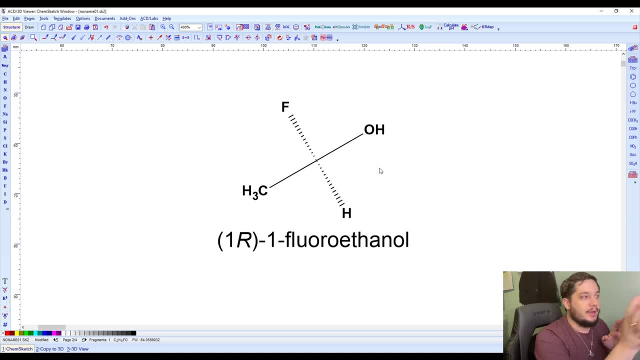 Um, but if you're getting that warning, it does mean that there's something Going on right now that it can't tell the stereochemistry that you're trying to communicate. So just, um, make sure that you try to simplify things or work with the software to make it a little bit more clear as to, oh, the your intended configuration. 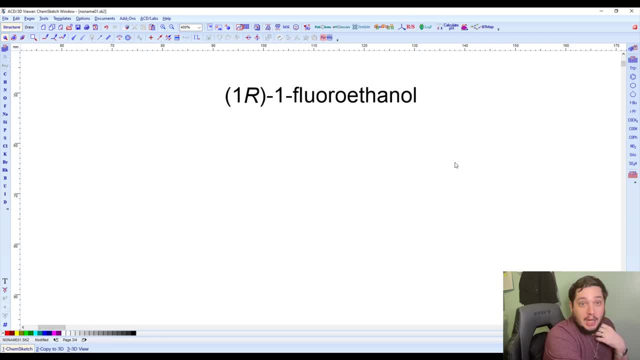 Now what if you have the name but not the structure, um, can the software do this? And the answer is yeah, you get this. uh, you just uh click the text box That is um that has the name in it, using the text feature right here. 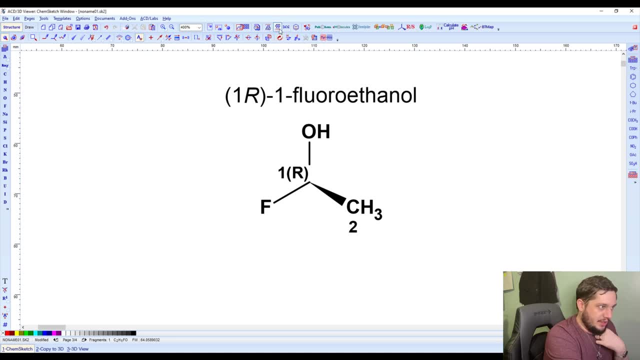 And then you can generate a structure from that using this button up at the top. Now you get, uh, these numbers, uh, that are attached to it too. Um, I don't like them as much, So I tend to remove them. but if you want them, that they're there for you. 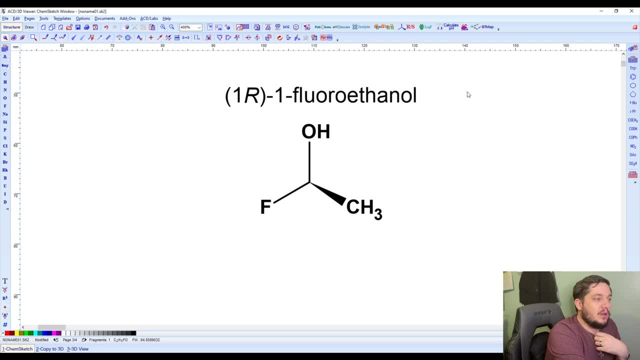 Um, so that's nice, And so that that is, uh, one of the other options that you can do, depending on where, where you're going and what you're coming from. Um, now the uh hydrogen here is attached. 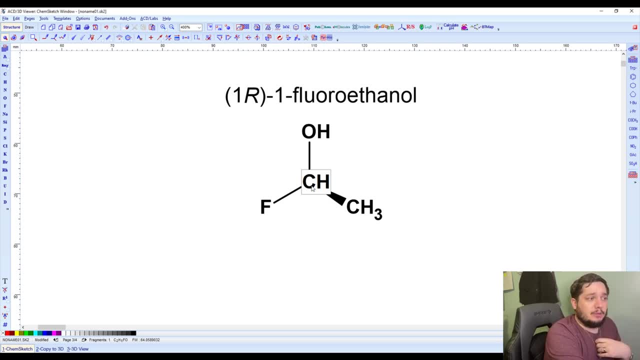 So the carbon is not shown in this structure, but it's sort of assumed that it's going into the back of the page um, which is a pretty normal convention with a lot of uh hydrogens that they just uh get, uh, you know, pushed to the to the back. 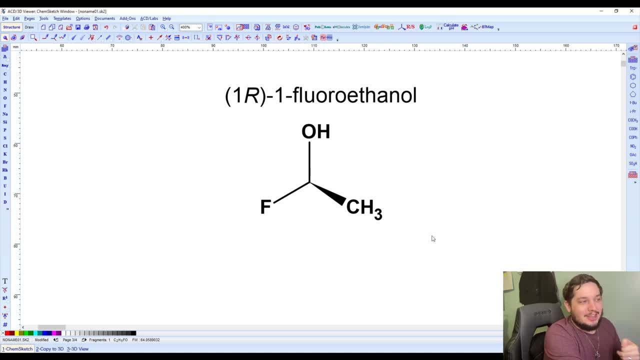 They don't get the respect that they deserve. Um, but uh, yeah. so that's something that you can be, um, you'll, you'll see sometimes if you're trying to generate the structures in this way. Okay, And then, lastly, I want to show you a the the more advanced version of the 3d view. 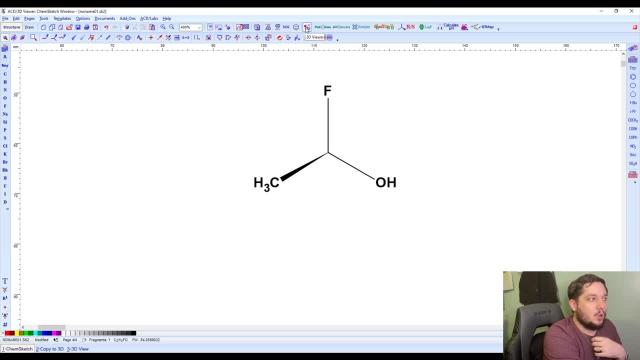 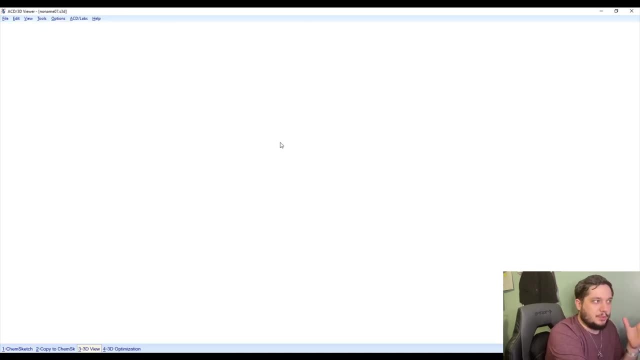 Okay, Because they think they're the this tool here. the 3d viewer is a really neat and is really helpful for um seeing the the the structure more holistically and getting a really in-depth view as to how things look. 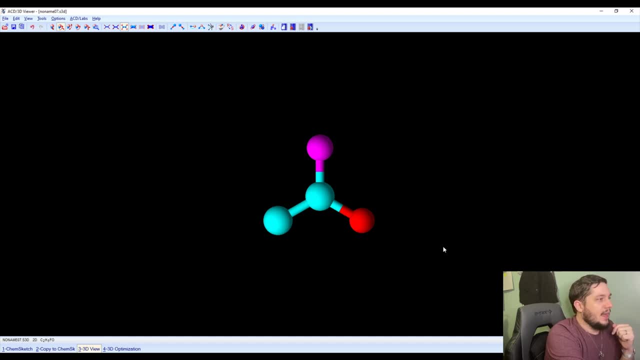 Um, this layout: here we have a black background and the the, the atoms. here we can, um, rotate things in three dimensions by using these tools. Now should note that the 3d viewer Viewer is slow, uh, relative to a lot of other things that happen in kind of sketch game. sketches generally gave, I think, a pretty fast program. 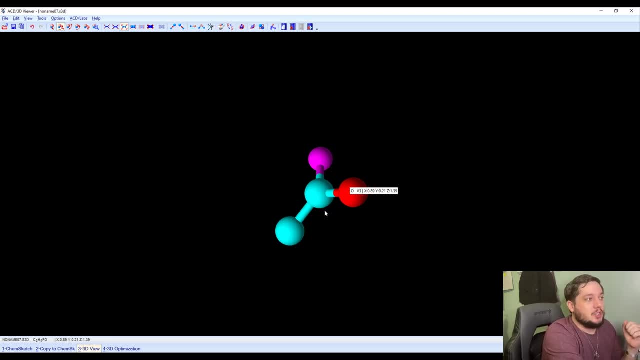 Things happen. you know more or less, you know instantaneously as you are doing things. Um, this is uh going to be the one area that it takes a little bit more time for it to figure things out. So if it is giving you some attitude, uh, be patient. 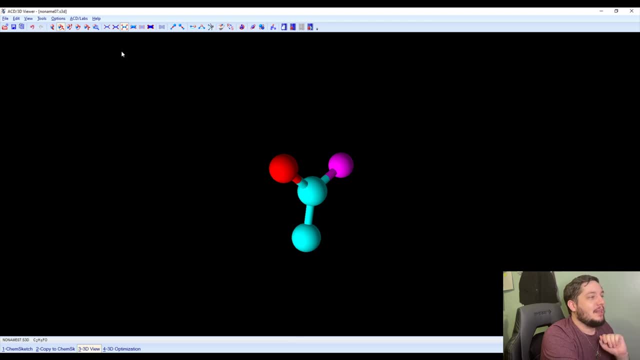 It's not just you know some problem with your computer, for example, Um it, it happens pretty frequently. Um, now we can do. the stick model Here is: uh, maybe it'll show things. Yeah, we have that. 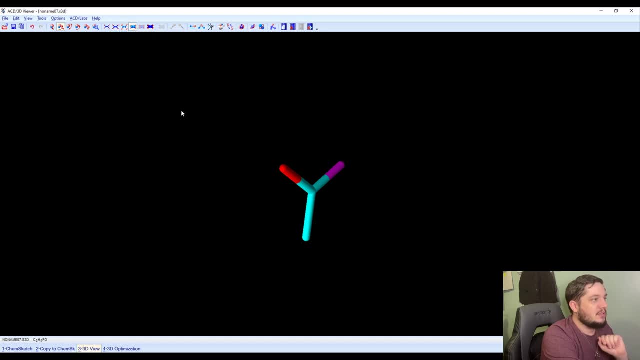 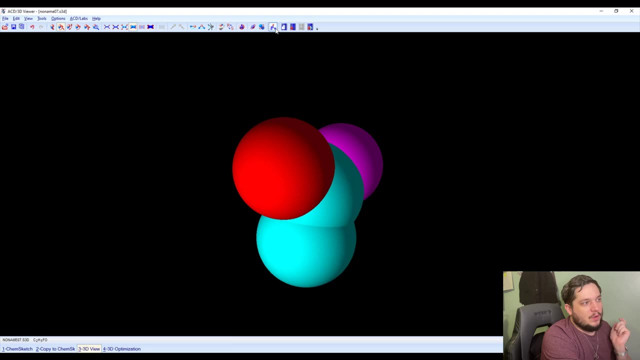 We have a different views. so that's balls and sticks. We have space fill, We have viewing things. Um, yeah, so we have all of that. Now, if we go ahead and we do the three optimization here, um, we're often going to see the hydrogens pop out too, because that was something that is important in doing the 3d optimization of the you see these in space and that it computes those in space. 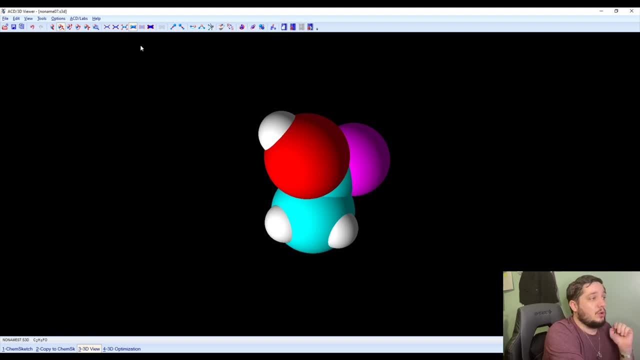 So that's something You should. uh, you'll be aware of too. That's a way to get them If that's something that you're looking for in it. uh, and you can see that layout, but we can. actually, I prefer the um, the ball and stick view in order to see the stereo chemistry the most clearly. 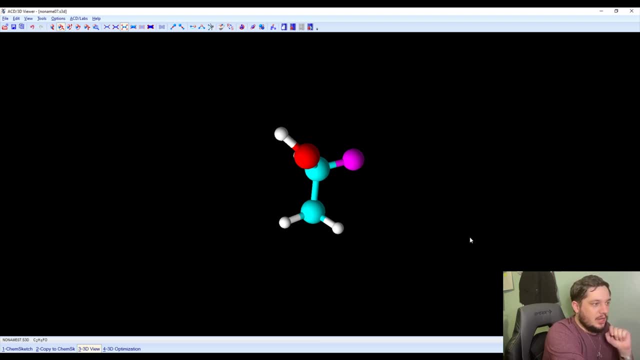 Um, so this is a little bit uh blocked right here, so I'm just going to turn it a little bit and then you can uh hopefully see things a little bit more clearly. Okay, That's, that looks pretty good. 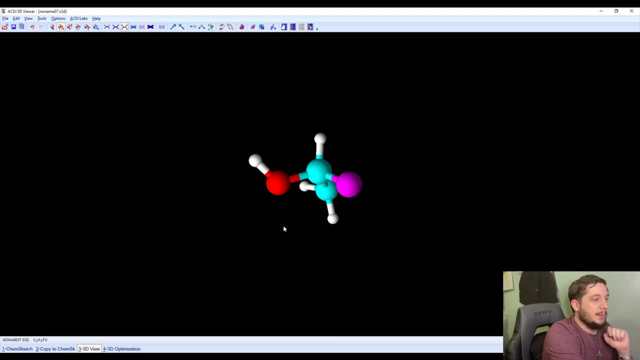 Yeah That, that is a pretty clear configuration that you can uh look at. You can uh look to see where the different groups align up to each other. but one function that is actually really useful is the invert center one, and this is for inverting the R and S configurations. 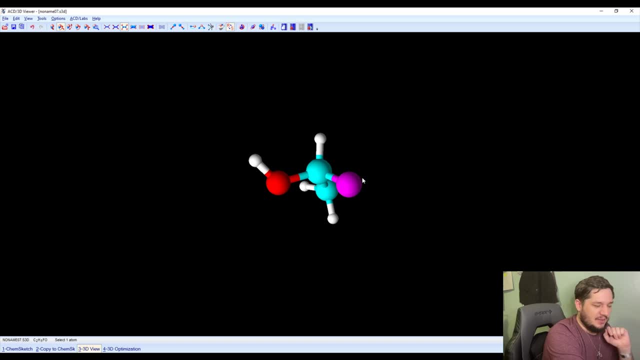 So when we click this here, we will go from the. I believe it's a um S configuration as of right now. Um, but we can go to the uh R configuration when we use this tool. So, yeah, we've, we have uh, flipped it around uh here, which is, which is good. 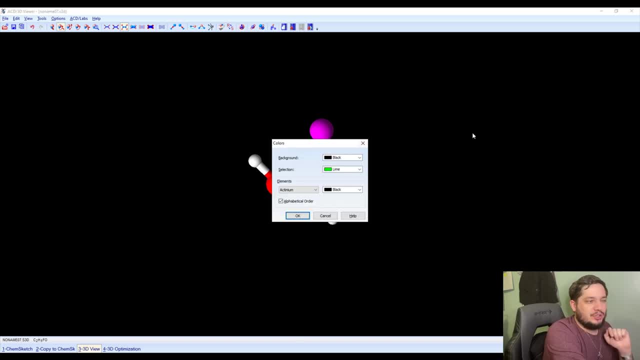 Um, but, And then you also have access to uh setting colors to you, So there's lots of things that you can do in terms of, um, changing the way in which, uh, everything looks. I actually prefer the- um, the grayish background, uh, not quite as heavy as the black. 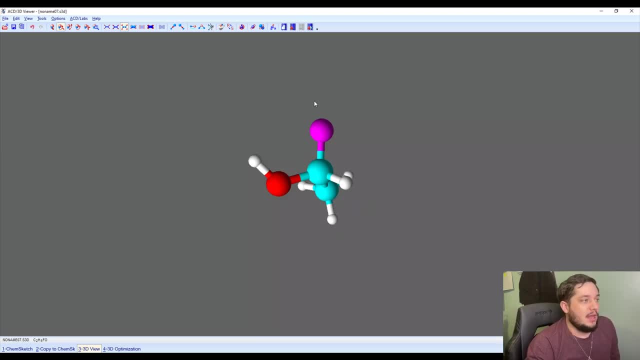 Um, so that's something that you can do as well. And, uh, if you want to do a lot in terms of, uh, looking at molecules, there are lots of options here that you have access to in order to kind of get you know everything that you want in. 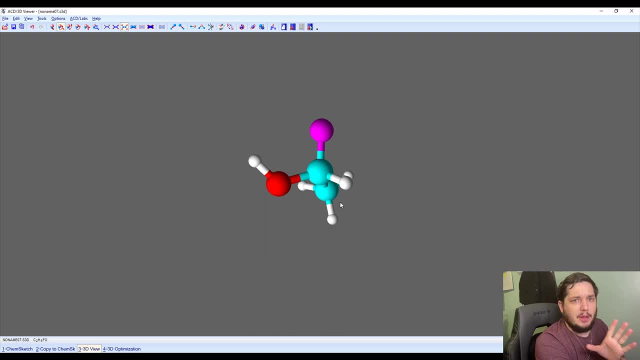 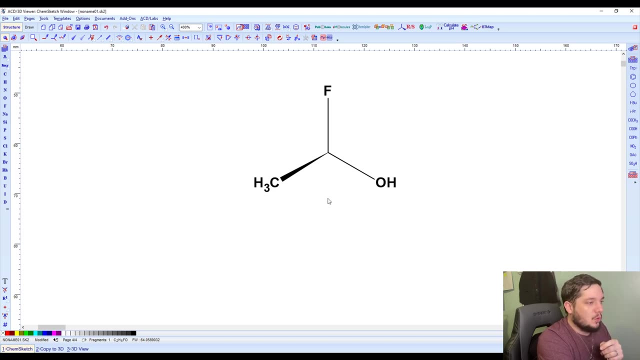 terms In terms of having your molecule looking great, but I think that that'll be it for today. Actually, one of the last thing to to mention, we can go back here and see our uh molecule once again in regular form.